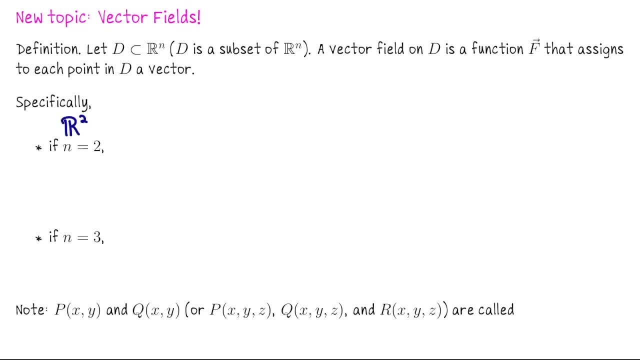 So how we denote this, if we're working, say, in R2, is we write: vector-valued function f of x and y is equal to an output which looks like a component function: p on x and y, q on x and y. So these are vector-valued functions, like we've seen before with curves, but the 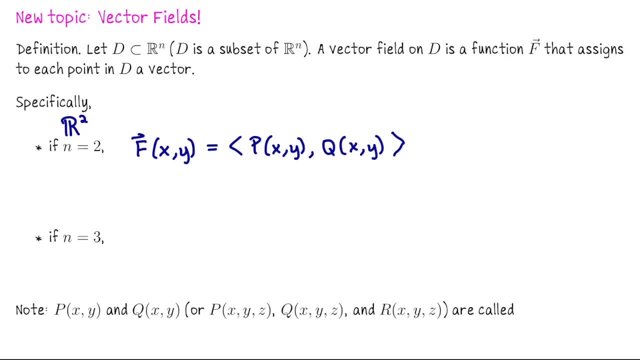 difference here is that the function is of multiple variables. In particular, to a point in R2, it associates a vector with two coordinates. Similarly, if we're working in three-dimensional space, our vector field would look like f of x, y. 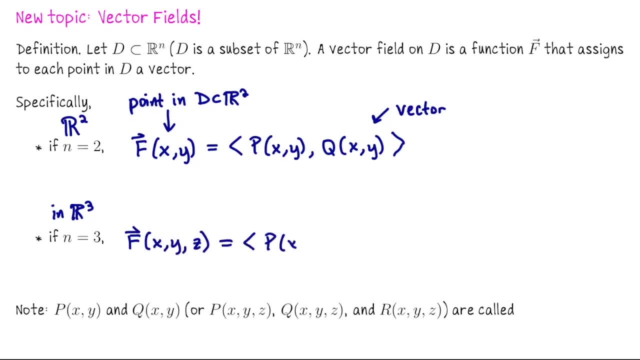 and z gives us a three-dimensional vector whose component functions would be p of x, y and z, q of x, y and z and r of x, y and z. If we look at the previous vector-valued functions that we've seen, we can think of p and q. 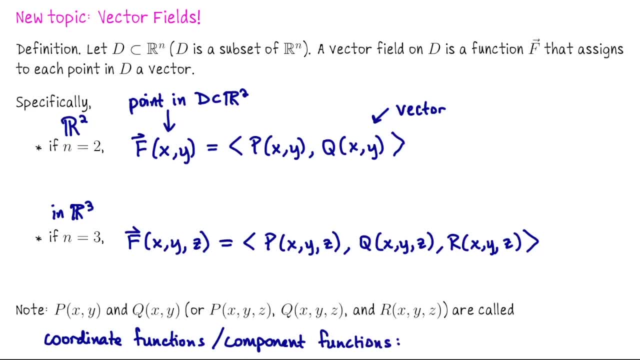 or p, q and r as coordinate functions or component functions, which associates to each point in D a coordinate. In other words, each component function is a scalar-valued function of multiple variables. The important thing here is the big picture. A vector field is a way of saying at this. 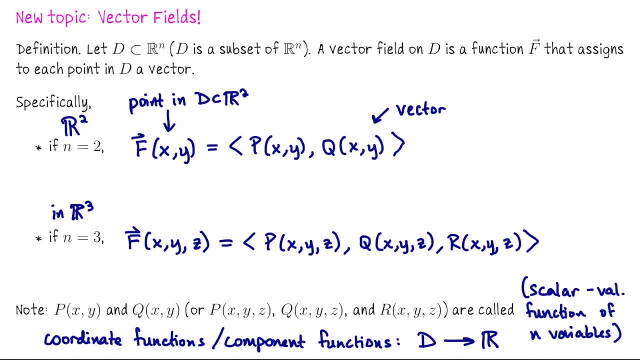 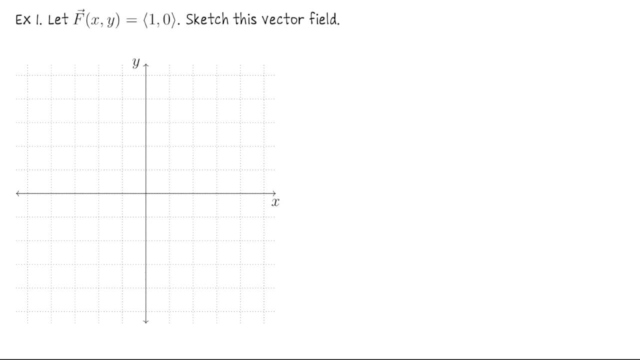 For our first example, let's look at. the vector field f of x and y equals one-zero. This is a vector field in R2.. Its domain is the entire x-y plane And what this vector field says is to each point x, y and r2, and then the vector field f of x and y equals. 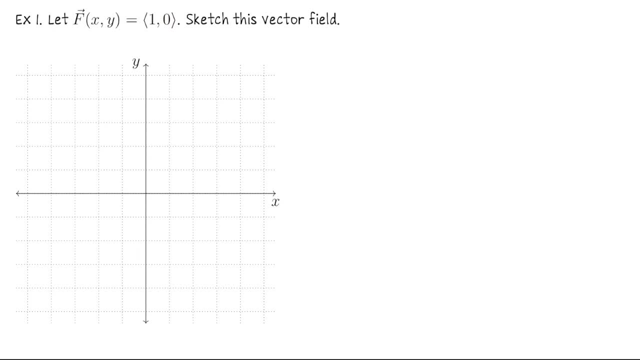 sketch the vector. So we imagine going to each point in R2 and attaching a vector that looks like: just go one coordinate to the east. So let me sketch a few of these. For example, if I come to the point I'm going to attach the vector. 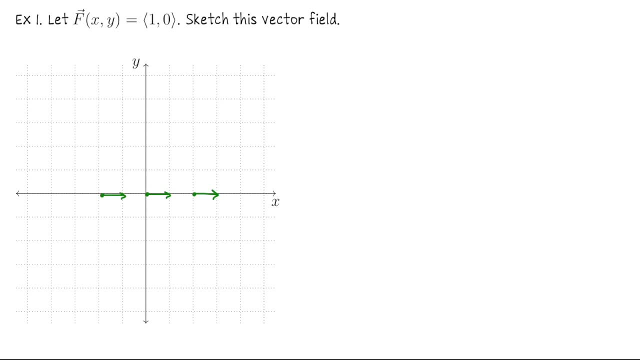 If I come to the origin, I'm going to attach the vector. Same thing if I go left on the x-axis, To every point I associate the vector. one unit to the right, zero units up or down. We can go up the y-axis. 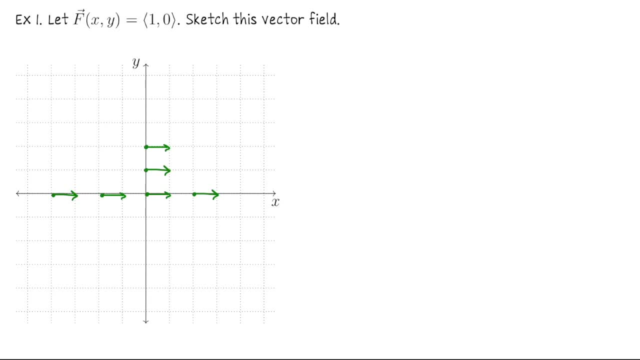 To each point on the y-axis I attach the same vector and you can see what we're going to do in the rest of space. At every point in the xy-plane I imagine attaching the vector. It's not a very interesting vector field. 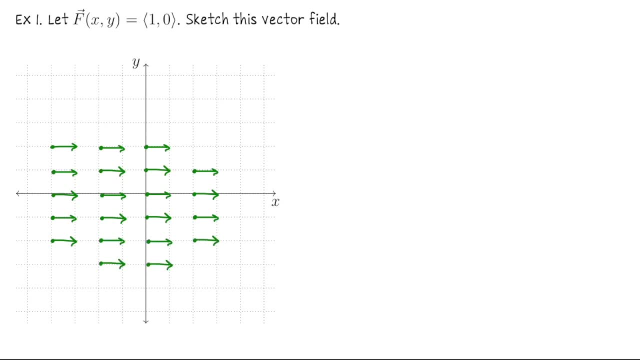 Everybody looks the same. Now, when I illustrated this vector field just now, I chose the points so that they're fairly spaced apart And in fact all of my xy coordinates here are grid points, But to every single point in R2,. 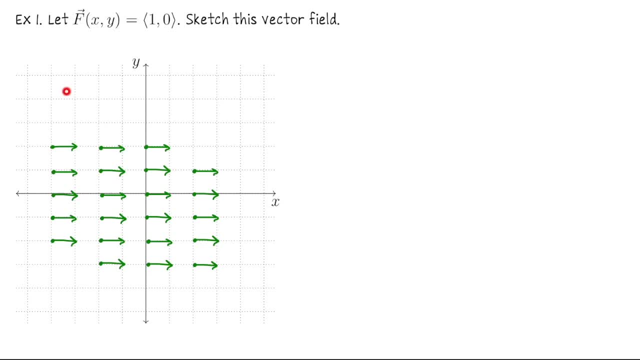 we associate the vector, Which means if I just pick this point right here, not a whole number for x or y, I would draw the same vector. So if I wanted to be overly detailed instead of just picking these four anchor points on the x-axis, 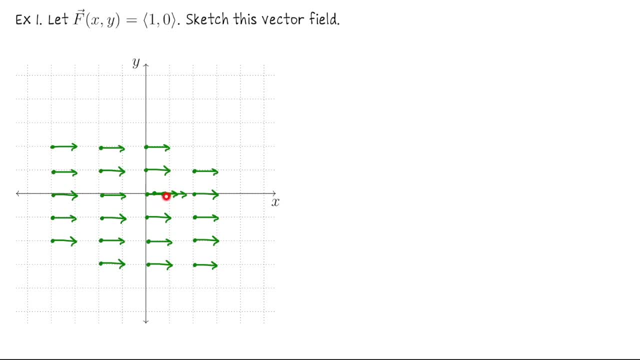 I could try to fill in at every single point between, say, zero and one. Just imagine drawing one zero for every point there or every point here. We would have a lot of overlap. So when we illustrate these by hand or by using some numerical software, 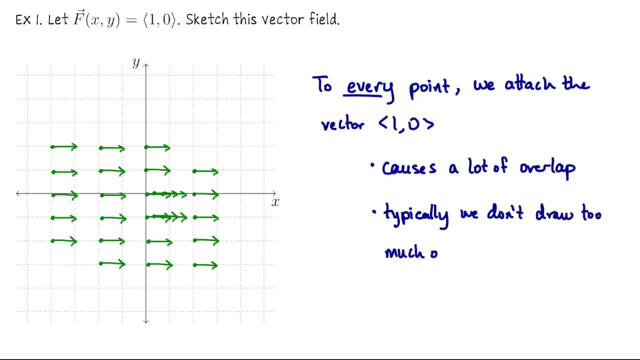 typically we don't draw our vectors as overlapping this much. We pick a nice set of points to illustrate the general behavior of the vector field. If I'm looking at this vector field, I get the overall picture. The picture is that this vector field points us to the right. 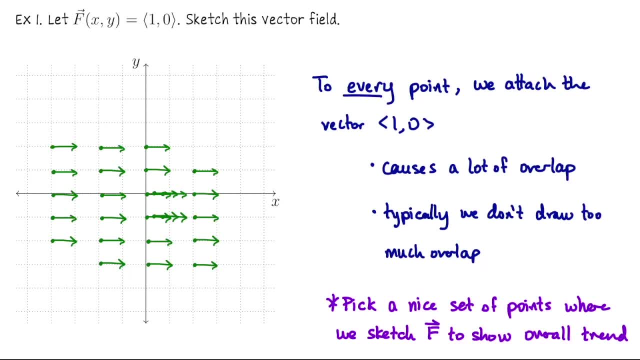 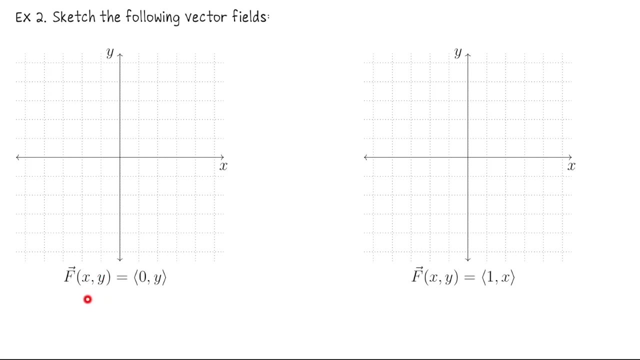 If this were a map of wind or fluid flow, I would understand the behavior of the fluid. It's flowing evenly to the right. Okay, let's look at a few more examples. Suppose f of x and y is the vector field that takes any point: x, y and r2. 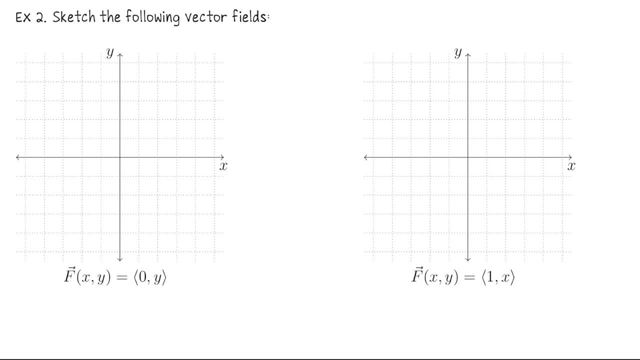 and attaches the vector zero y. Let's see what this vector field looks like by just plugging in some points. So how about we start with the origin f of zero? zero is zero, zero. So there's that vector. It has no magnitude. 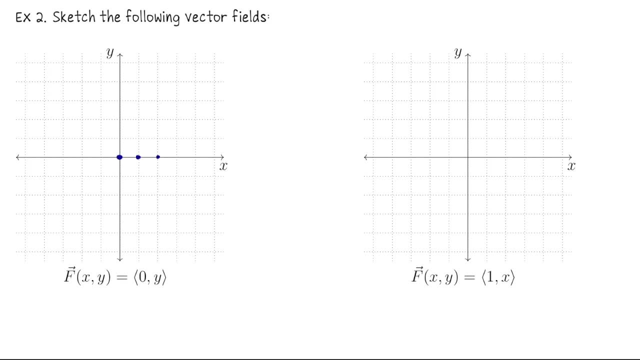 In fact everywhere along the x-axis, because the y-coordinates along the x-axis are zero. to every point on the x-axis we would associate the vector zero- zero. So for every point on the x-axis, I'm going to sketch this vector. 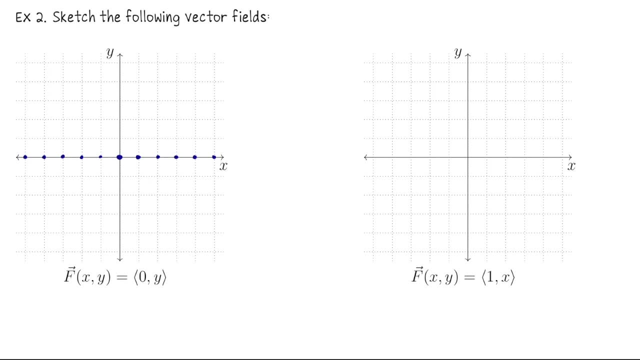 And, as I mentioned a second ago, we're not only interested in the vector at integer values of x. we could fill in the x-axis like this, But it's unnecessary to give this many examples, right Once we see the trend behavior. 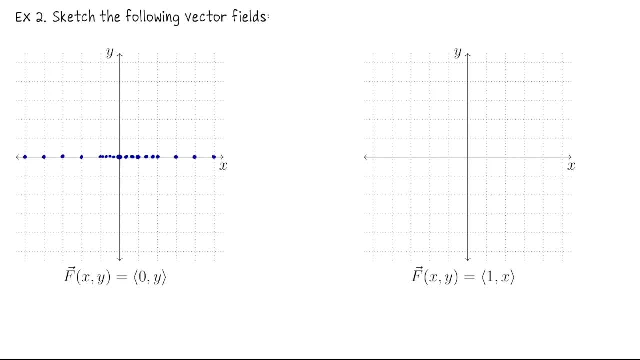 we can go on to other regions and the x- y plane. So what happens? if I say: go down to the third and fourth quadrant, The vector we attach to any point has no dependence on x. So every vector would point either north or south. 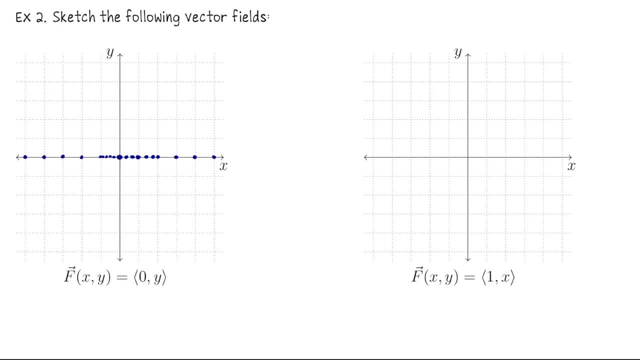 There's no east-west component, It's just zero in that first coordinate. And then how much it points north or south depends on the y-coordinate. So if I come down to y equals negative one, every single vector is going to look like zero negative one. 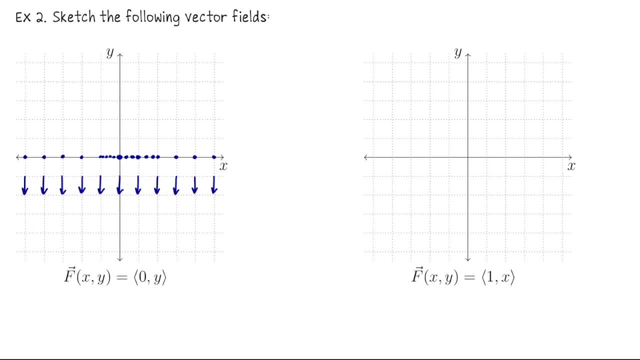 So to each point at the level y equals negative one, I sketch the vector zero negative one. To every point x, y that has y equal to one, I would sketch a vector that points one unit north. And then same story if y is negative two. 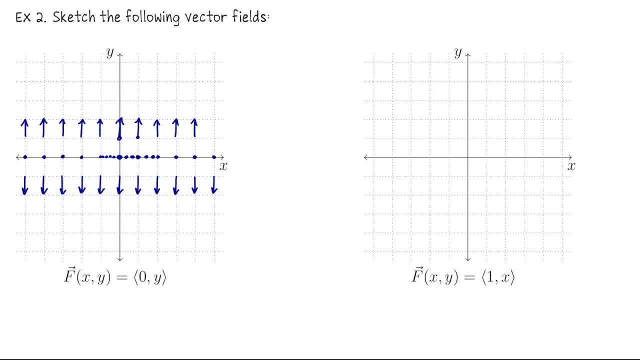 every point that has a y-coordinate of negative two is going to get the attached vector zero negative two. So we can fill in our vector field like this Up here: y is three. To every vector we attach the vector zero three. 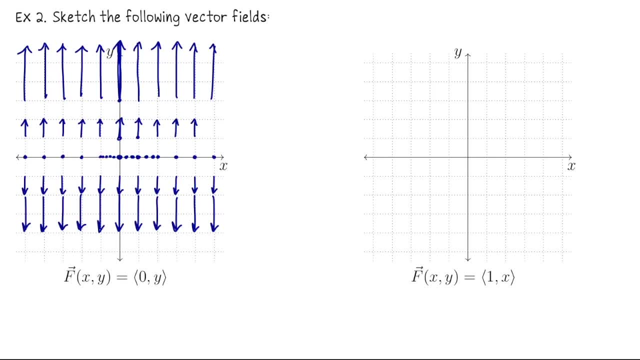 So this is a picture of this vector field. Now imagine this vector field was modeling some motion. If I dropped a piece of confetti right here, what would happen? It would start to move up, and then we get the feeling maybe it's going to move up at a faster rate. 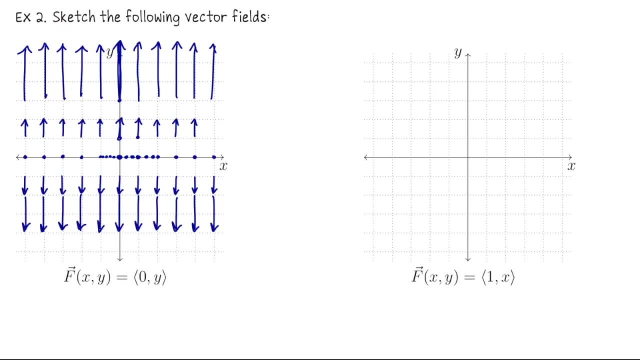 because the arrows get taller. So this is giving us our sense of motion. If I dropped a particle right on the x-axis, it wouldn't move at all. If I dropped a particle down here, it's going to flow down. Okay, let's look at the vector field. f of x and y equals one comma x. 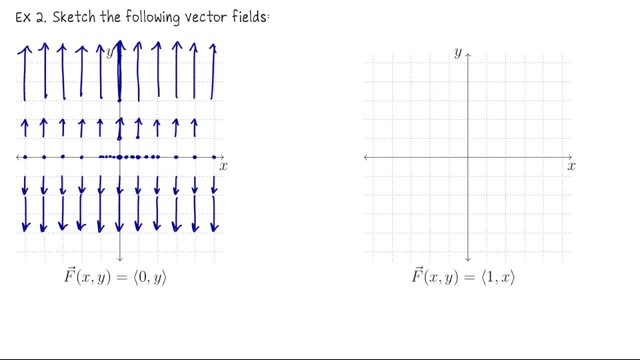 Start with the origin f of zero. zero is the vector one zero. Let me go down to the point: zero negative one. The x-coordinate of zero negative one is zero. So this vector will also be one zero. In fact, we see that up and down the y-axis. 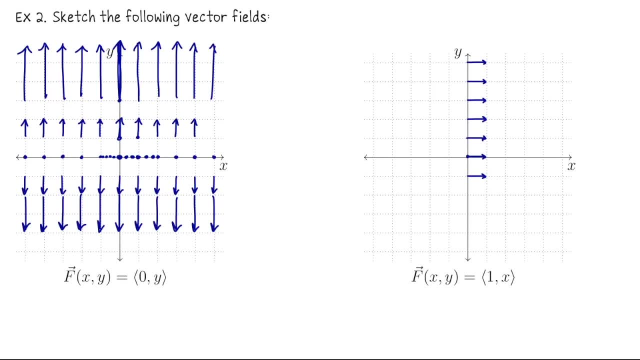 we're going to attach the vector one: zero. Okay, let's come over here to this point. One negative one. The x-coordinate is one. So at this point I'm going to attach the vector one one. One unit east, one unit north. 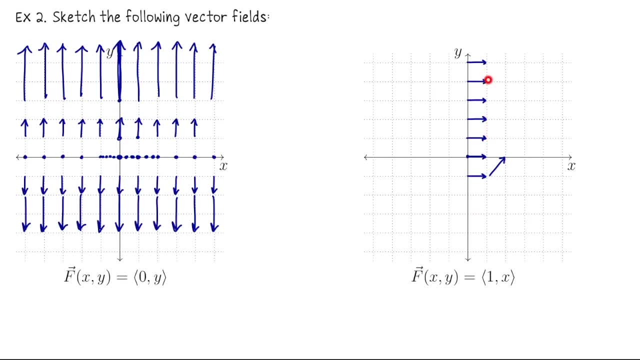 And then if we go up and down again, we see that every coordinate that has an x-coordinate of one is going to get the same shape: vector One east, one north. We can draw a bunch of vectors like that Go over to the other side. 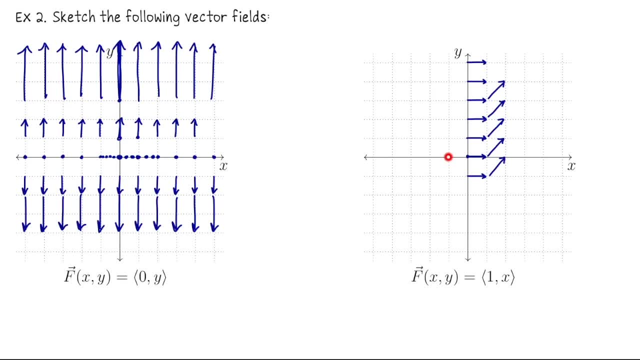 Let's say we're at the point negative one, zero. The x-coordinate is negative one. So this vector is going to be one negative one. That's one unit east, one unit south. Then we can go up like this, Okay, and we can fill in the rest of the plane like this: 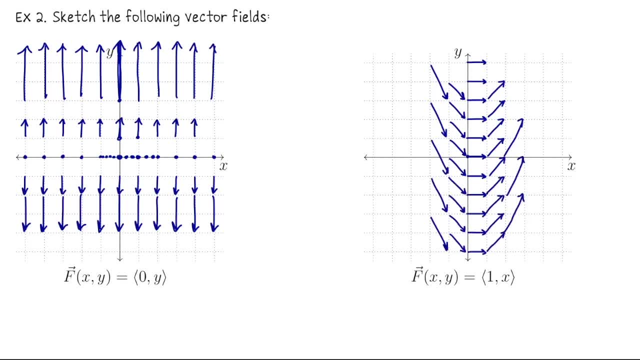 just to give a sense of motion, Suppose this is modeling a fluid and I drop an object right here. How would we expect that object to move based on this picture? Well, according to the vectors, it's going to go down a bit. 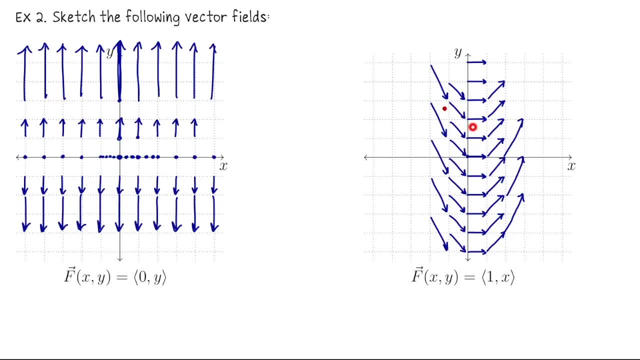 but then once it gets here, it's going to go straight to the right and then it's going to turn. So we can imagine a sense of motion built into this vector field. Same thing if I come down here Again, we're going to go down flow to the right. 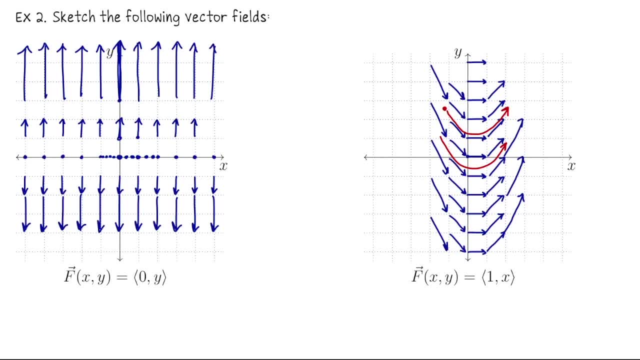 and then turn and flow up, kind of like that. This is a vector field I drew by hand. Again, when you draw a vector field by hand, you do the best you can to give an overall picture of the behavior of the vector field. 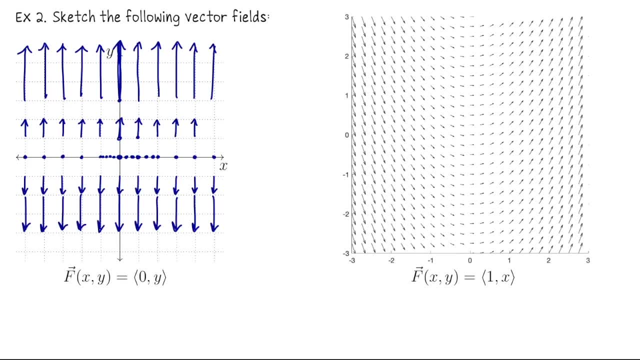 Here's an image of this vector field. Here's an image of this vector field produced in MATLAB. Using software can be a great way to generate a much larger picture of the vector field. Notice that, while MATLAB is doing a great job with the sense of direction, 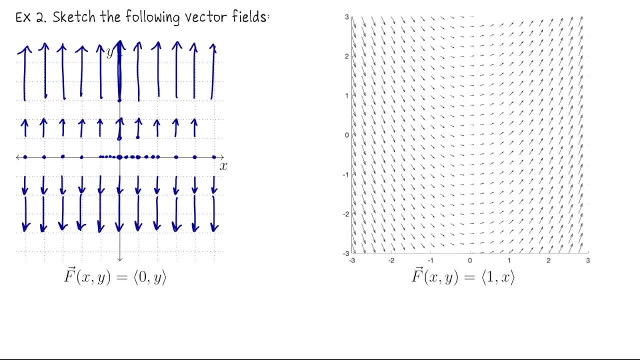 the magnitudes of the vectors might not exactly match the magnitudes that we sketched by hand, And that's because it's common for software like this not to give necessarily the true magnitude of the vector at any point, but rather a relative sense of that vector's magnitude. 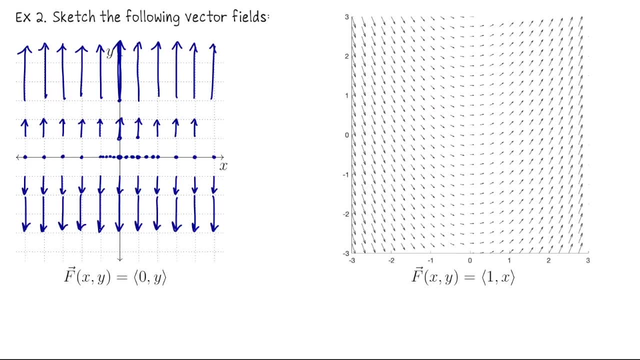 compared to the rest of the graph. So here the magnitudes are more relative to each other, kind of scaled to give a good picture of the behavior of this vector field. that's not too messy with too many overlapping vectors. So often when we generate a picture of a vector field, 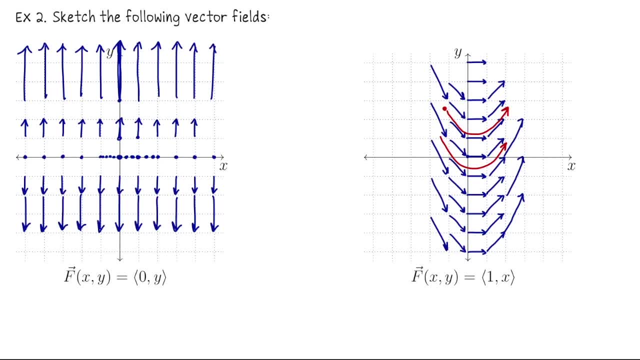 whether it's by hand or with a computer. sometimes we don't care too much about the magnitude of the vector, because what's most important is the sense of direction, And you can imagine if you kept drawing vectors like this. they would become so long that they would overlap. 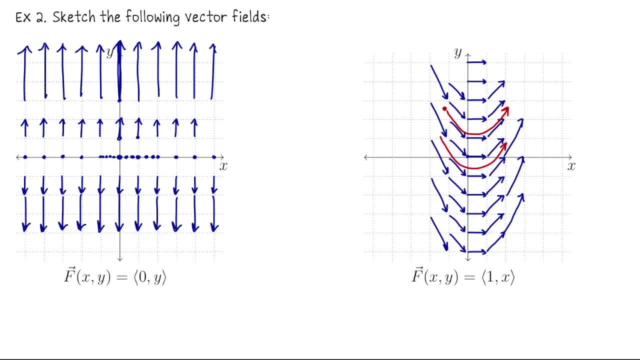 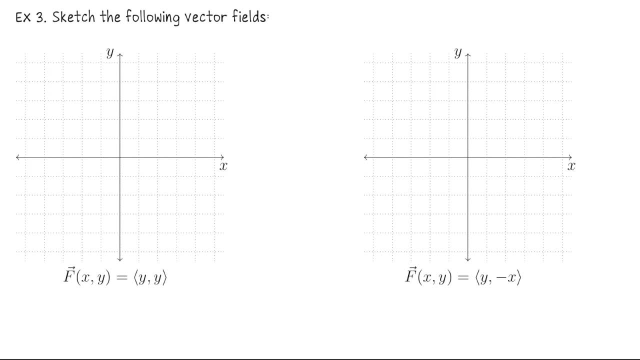 and make the picture kind of messy. Let's finish with these two examples. We just want to sketch these vector fields in R2.. The first vector field says: to any point x, y in R2, attach the vector which is the y-coordinate. 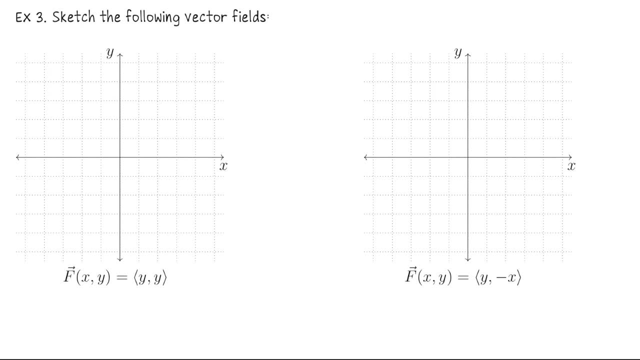 comma, the y-coordinate. So if we're at the origin the y-coordinate is 0, so we would attach the vector 0,, just a point. And then we realize, oh wait, all along the x-axis it's going to be the same story. 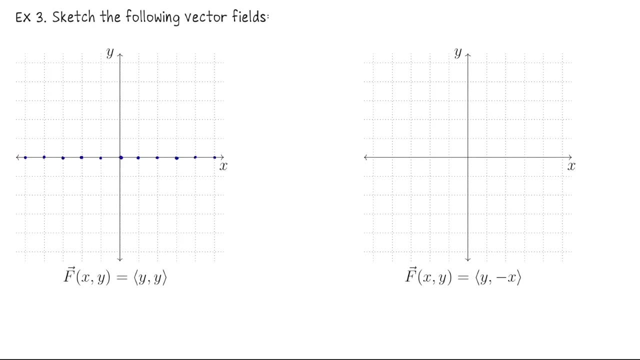 Because for every point on the x-axis the y-coordinate is 0, so to every point on the x-axis we attach the vector 0, 0.. You can now imagine I'm at this point- negative 3, 1.. 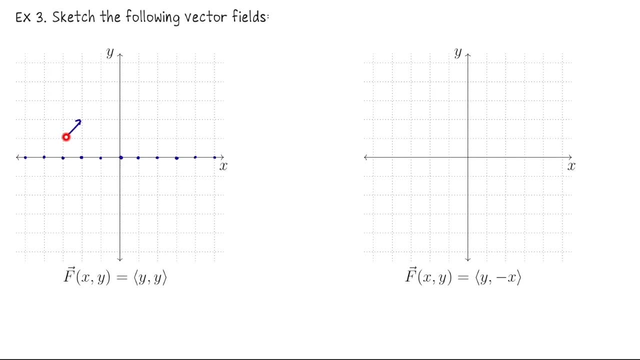 The y-coordinate is 1, so we attach the vector 1, 1.. Similarly, if I'm at this coordinate negative, 2, 1, the y-coordinate is 1, so once again, we attach 1, 1.. 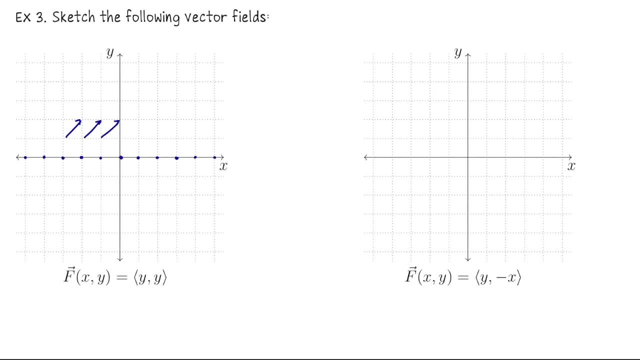 And we say, wait all along that line. whenever y equals 1, we're going to attach the vector 1, 1.. What about at negative 3, negative 1? The y-coordinate is negative 1, so we attach the vector negative 1, negative 1.. 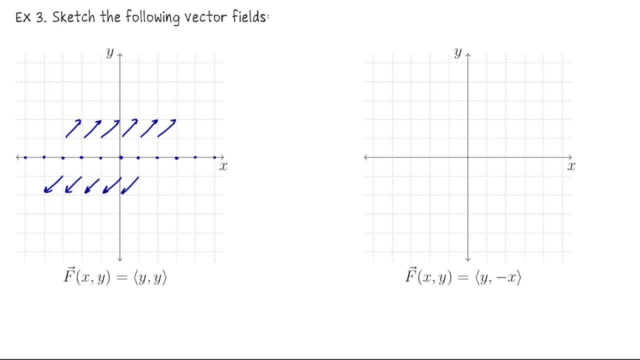 And same story: as we travel to the right, we keep attaching the vector negative 1, negative 1. Go up to y equals 2.. Any point that has a y-coordinate of 2, we'll get the vector 2, 2.. 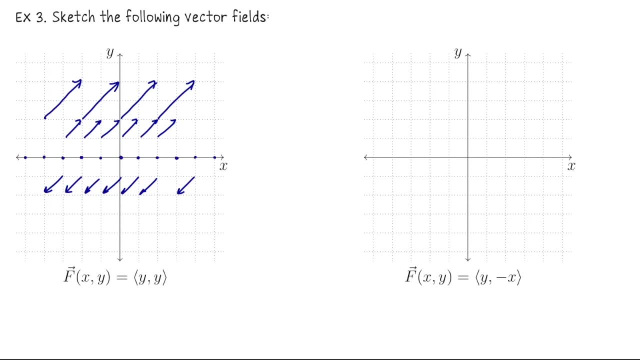 So here I'm still paying attention to the magnitude. so I drew this vector to be truly: 2 coordinates to the right, 2 coordinates up, Go down to any coordinate that has a y-value of negative 2, you get the vector: negative 2, negative 2.. 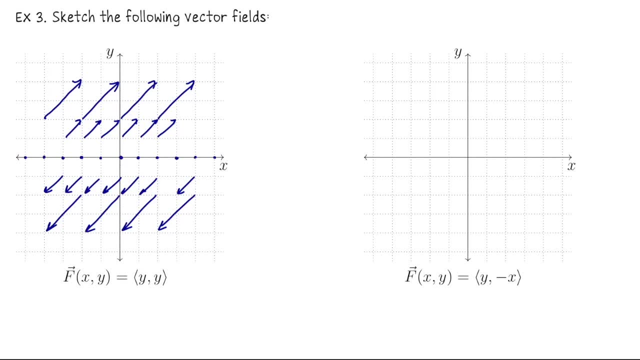 So overall, this is enough to get a feeling for the flow of this vector field. Okay, let's look at f of x and y. is y negative x? Start with the origin, that's going to get 0, 0.. 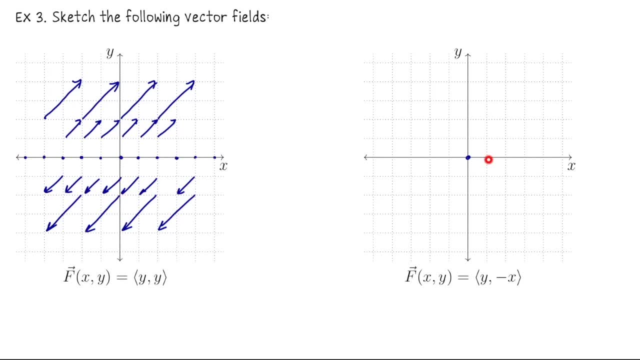 Okay, this one is easy to get kind of twisted around, so let's go real slow. If I come to the point 1, 0, I'm going to switch their coordinates and negate the second one. So 1, 0 is going to be 0, 1,. 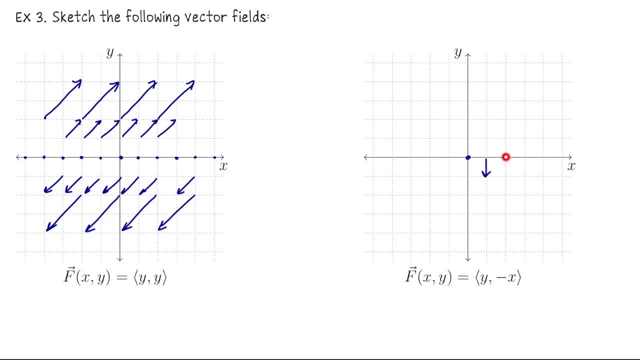 it's going to be 0, negative 1.. 2, 0 is going to be 0, negative 2.. Let's go to the left. Negative 1, 0 is going to be 0, negative 1,. 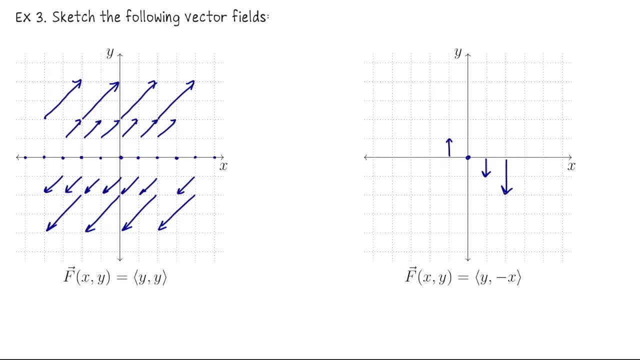 negate that second coordinate, that's 0, 1.. Negative 2, 0 is going to be 0, 2.. Okay, let's go on the y-axis: 0, 1 would be 1, 0.. 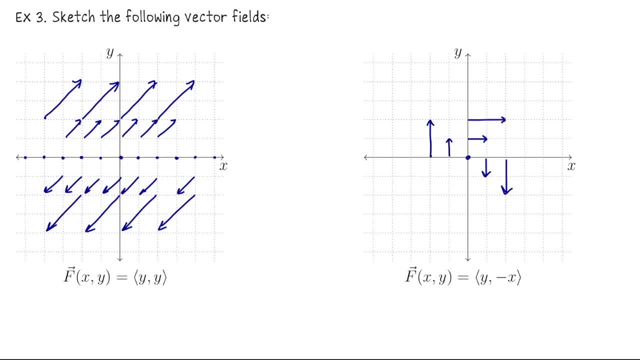 0, 2 would be 2, 0.. 0, negative 1 would be negative 1, 0.. And 0, negative 2 would be negative 2, 0.. Okay, let me pick a couple points. 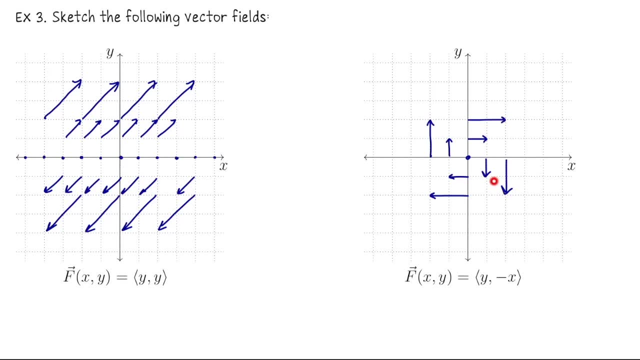 which aren't on the axes. Okay, let's do this. point 2, negative 1.. This one I'm going to have to write down. So f of 2, negative 1.. It's going to take the y-coordinate. 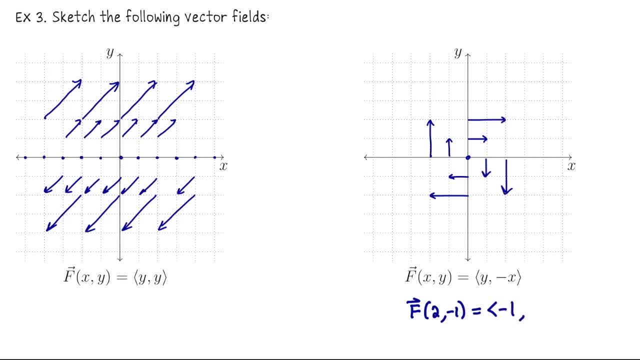 so that's negative 1, and then negate the x-coordinate, so that's negative 2.. So this is going to point in the southwest: one unit west, two units south. What about this point here? That's 1, negative 2.. 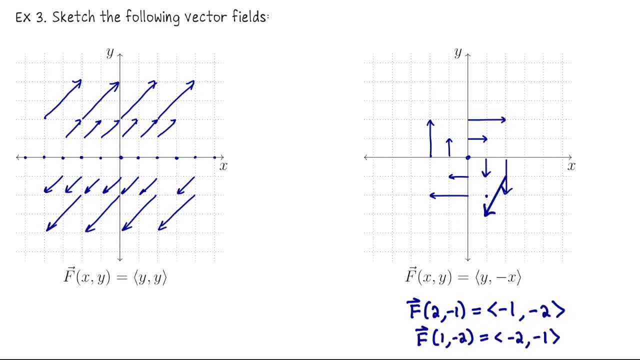 That's going to be negative 2, negative 1.. So that's going to point two units west, one unit south. This point here is negative 2, negative 1.. So that's going to be negative 1, 2.. 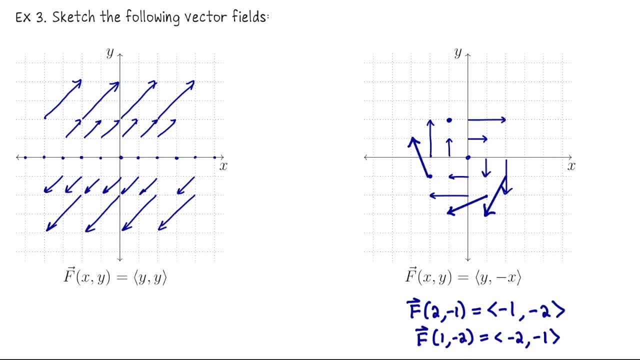 This point here is negative: 1, 2.. So that's going to be 2, 1.. Let's just do 1, 1.. That's going to be 1, negative 1.. Okay, that's probably enough to get a feeling. 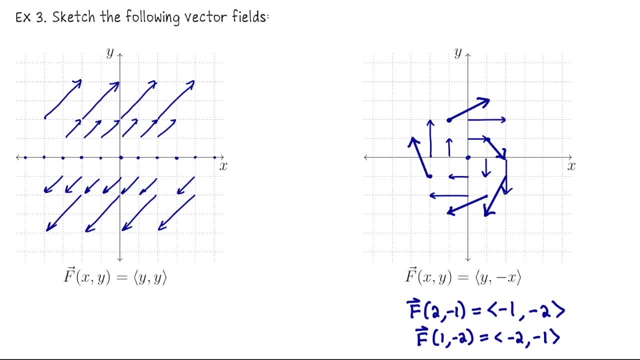 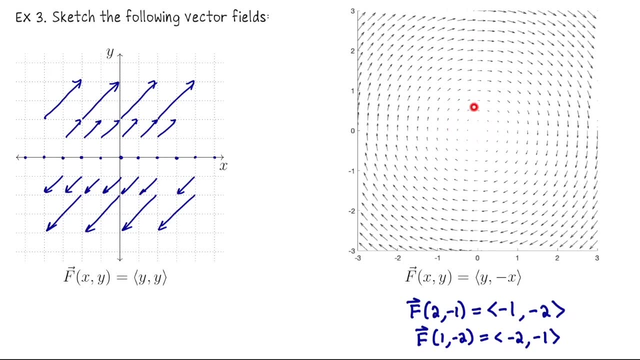 for this vector field. It seems to be revolving clockwise. Here's the vector field in MATLAB. You can really see the clockwise rotation. The vectors close to the origin have very small magnitudes. Those can be hard to make out. And once again, the magnitudes of the vectors. 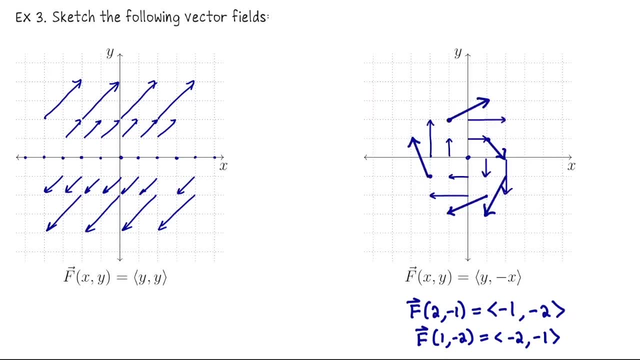 pictured in this graph have been scaled relative to each other. All of the examples that I sketched in this lecture were vector fields in R2, because that's the ones that are most reasonable to sketch by hand, even reasonable to do with a computer. 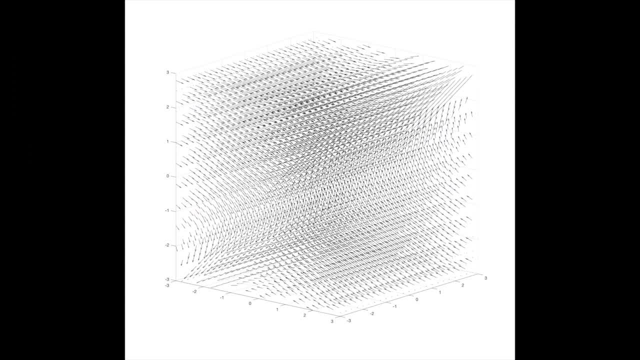 So here's a picture of a vector field in R3.. So you can see why I didn't try to sketch one of these by hand. So typically we won't illustrate these concepts in R3 because the pictures are very messy, But conceptually understand that a vector field in R3. 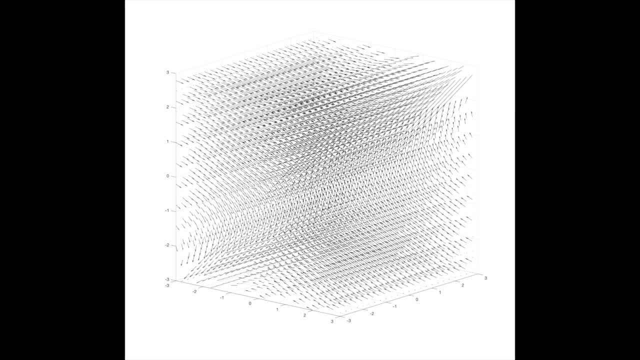 is going to take any point x, y, z in R3, any point in the domain of our function, and attach a vector which, of course, is going to have three components, so some amount in the x-direction, y-direction and z-direction. 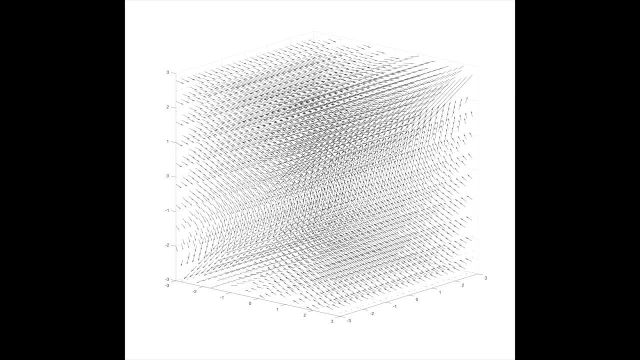 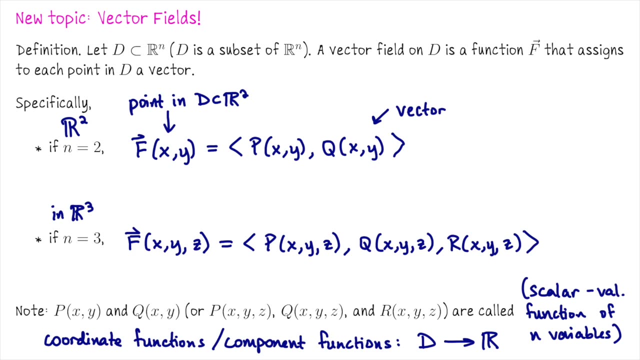 So, in particular, we could have something like a fluid volume, like a tank or a river, and we could model the direction of the fluid with a three-dimensional vector field. In this lecture I just wanted to present the definition of a vector field and how to sketch them. 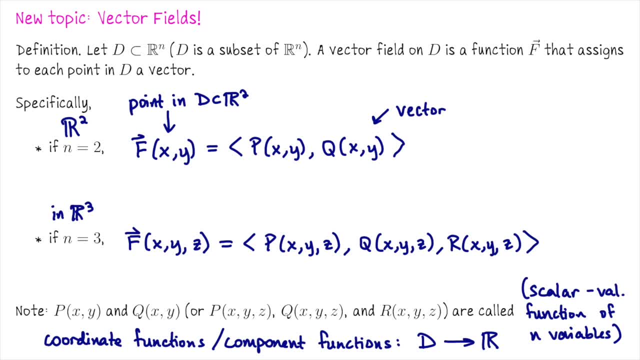 We have a lot to look forward to with vector fields. Thank you for your attention.